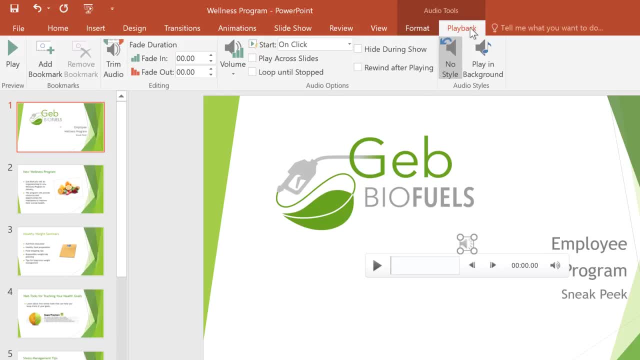 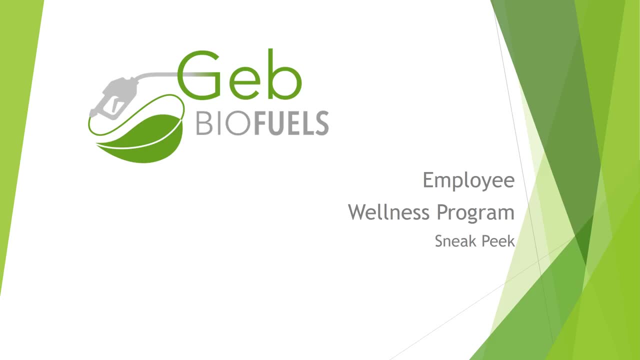 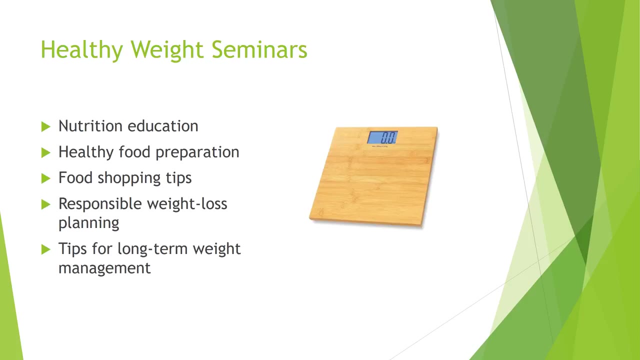 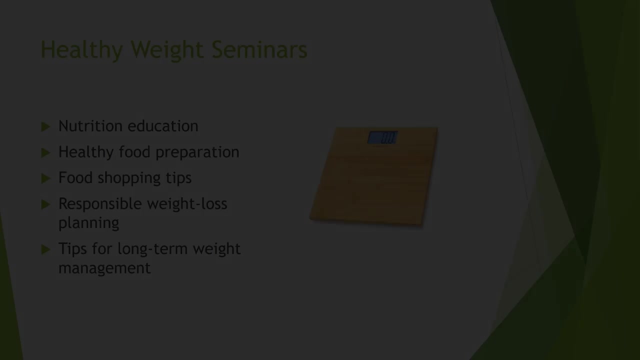 selected. make sure the Playback tab is open and then choose Play in Background. Let's start the slideshow and hear how it turned out. Now the audio plays across the entire slideshow. This trick can open up all sorts of new ideas for your presentations, so have fun experimenting. 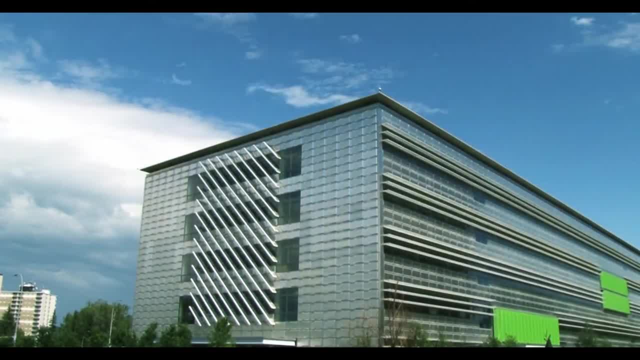 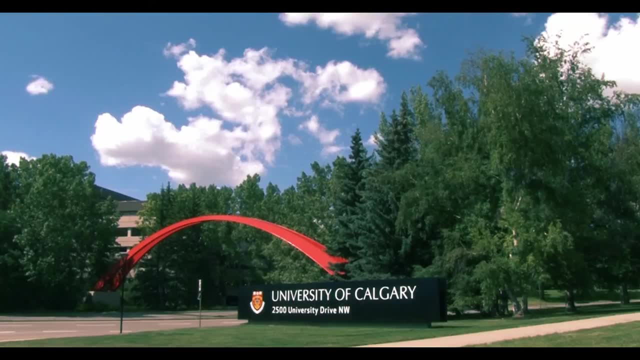 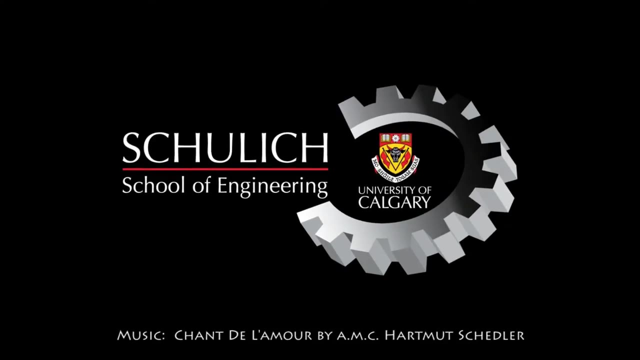 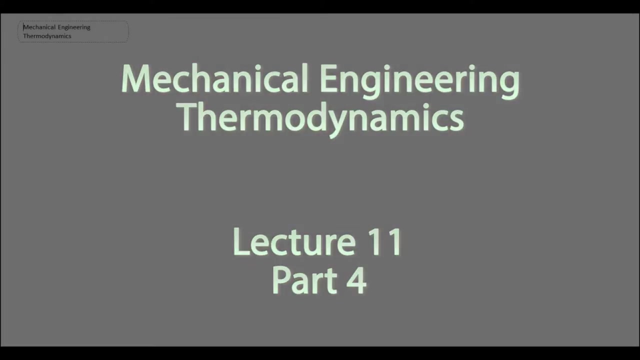 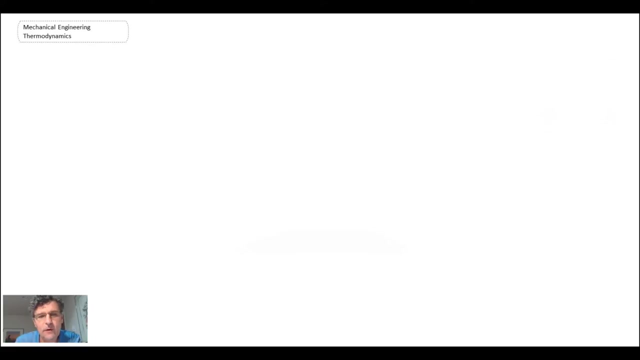 Now, when we're dealing with exergy and exergy analysis, one thing that we do need to consider is the amount of work that we are doing on the surroundings. So exergy itself considers performance with respect to a dead state. Exergy itself considers performance with respect to a dead state. 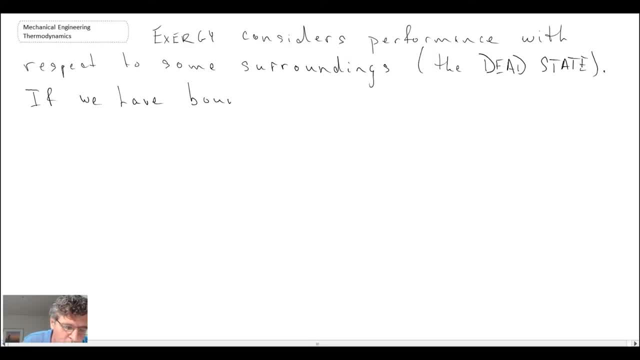